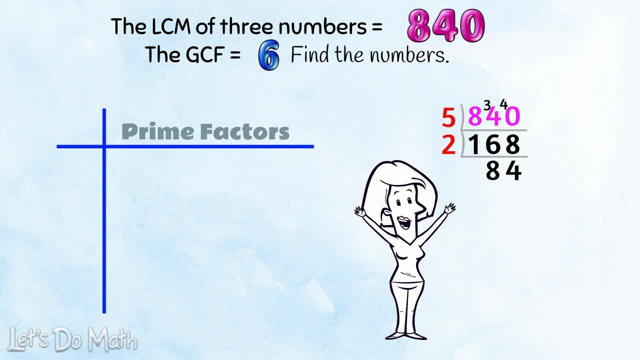 4 x 2 is 8: 84!. Great, We know that 7 x 12 is 84. So we can jump into Factor Tree mode to finish this off quickly: 84 is from 7 x 12.. 12 is from 2 x 6. 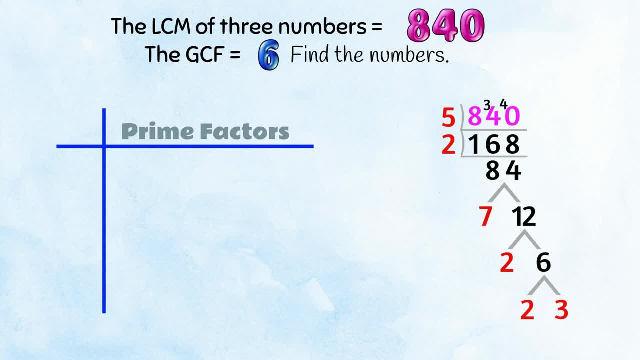 and 6 is from 2 x 3. Circle all the primes so you don't miss any. Then transfer the primes into the table, Set up the LCM line and write them here. We know the GCF is 6.. The prime factors of 6 are 2 and 3.. 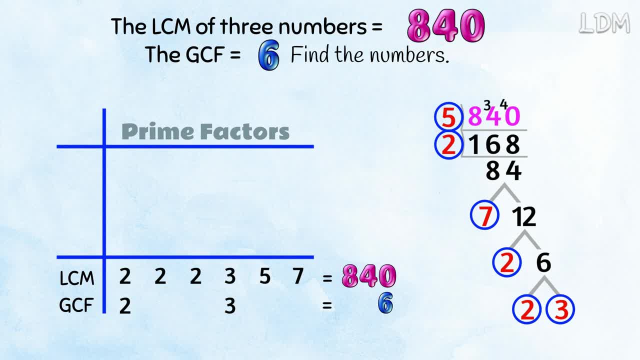 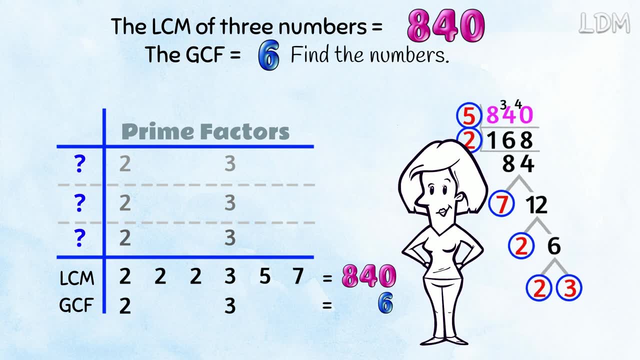 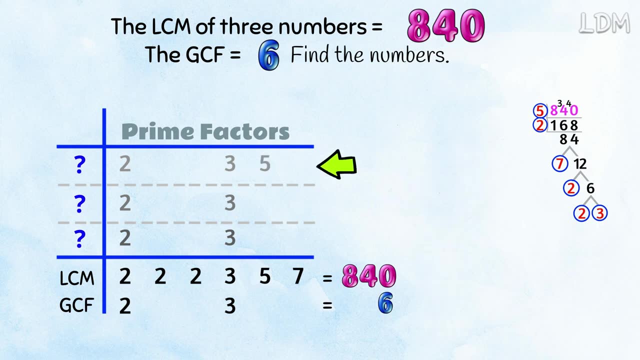 So they're the primes of the GCF. That means all 3 numbers need the primes 2 and 3.. And now we need to use the rest of the primes in some way so that the LCM line is true. Here I'm going to write 5 and 7.. 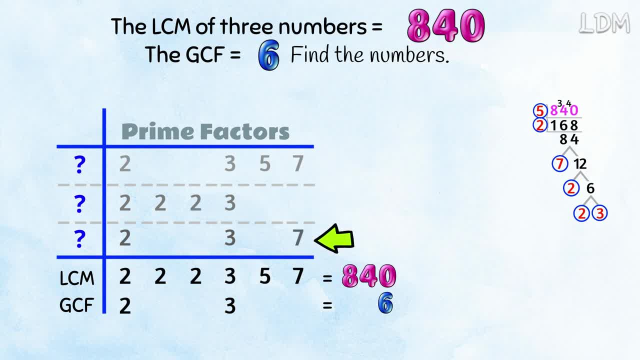 Here a couple of 2s And here a 7. Every column has at least one prime, but only the factors 2 and 3 are common to all our numbers, Because they're the primes of the GCF. Now let's find out what numbers we've got. 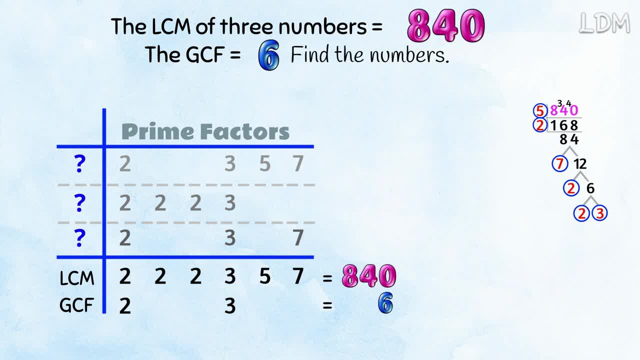 Multiply a row of primes to find the number. Here, 2 x 3 is 6 x 5 is 30 and x 7, 30 x 7, 3 x 7 is 21, and put in a 0, because we're multiplying by 3 tens. 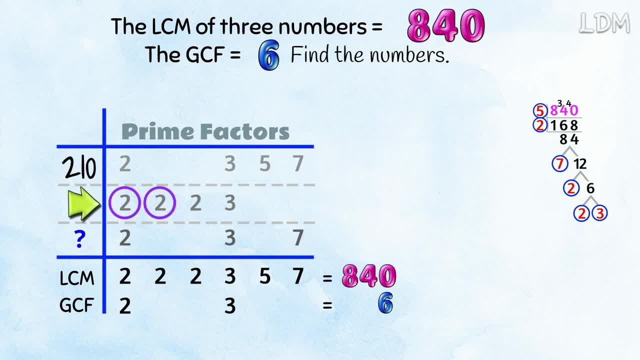 210. Next, we've got 2 x 2 is 4, x 2 is 8, x 3 is 24, and here 2 x 3 is 6 x 7 is 42. And there's my solution, Depending on how you spread the primes. 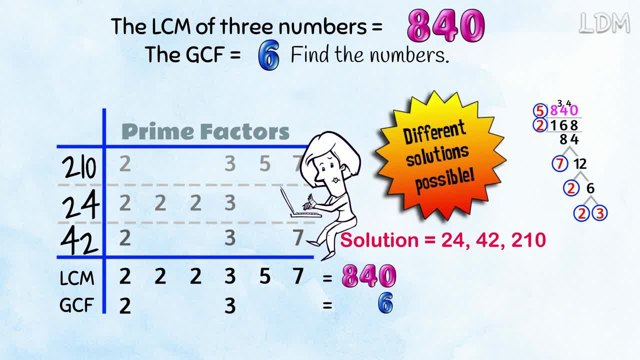 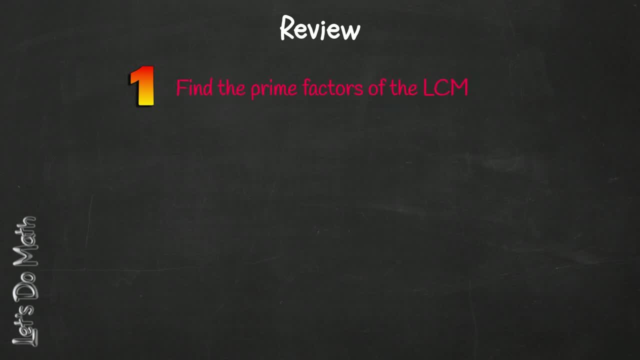 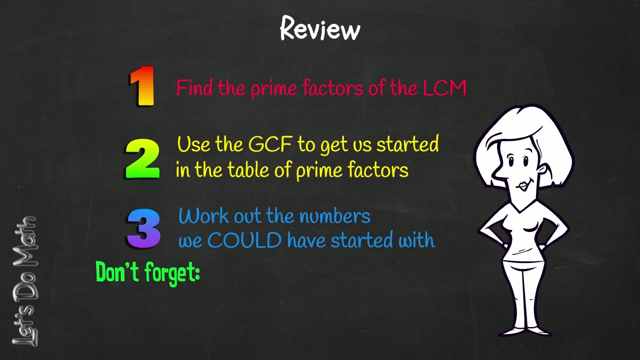 you'll get a different solution. There's a lot of possibilities here. Let's review for your notes, Let's work out the numbers we COULD have started with And at the end, don't forget to have a line that clearly states your solution numbers.